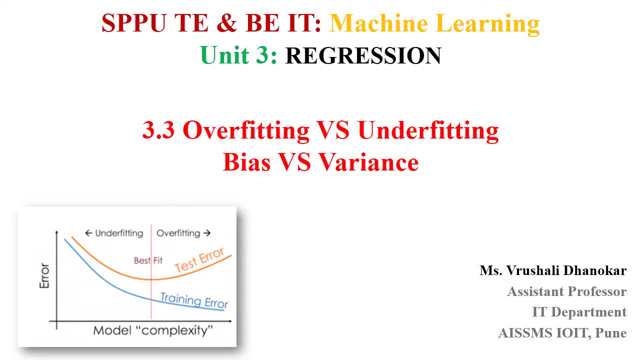 Hello everyone, this is Vrishali. In my last lectures we learned about Unit 1 ie- Introduction of Machine Learning, Unit 2, Classification, and also some points in Unit 3, ie- Cost Function, Concept of Regression List, Square Method. So I have mentioned the link of that videos. 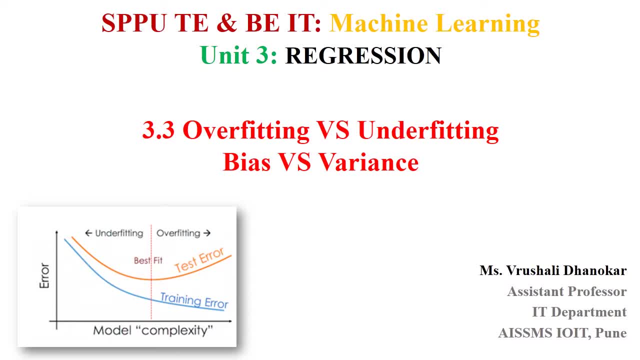 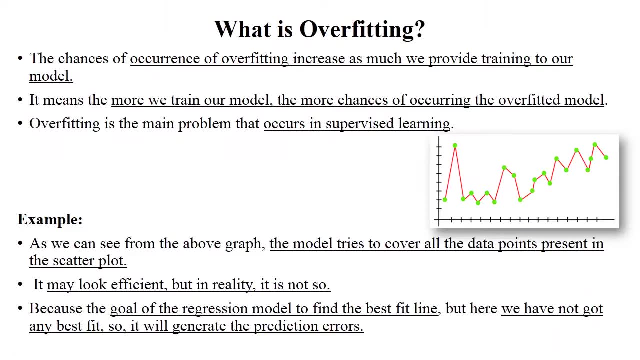 in below description box. So in this session we will learn the next concept, ie Overfitting versus Underfitting and Bias versus Variance. So let's see So, first we will learn the concept about what is overfitting. So basically, overfitting means, if you train your model, 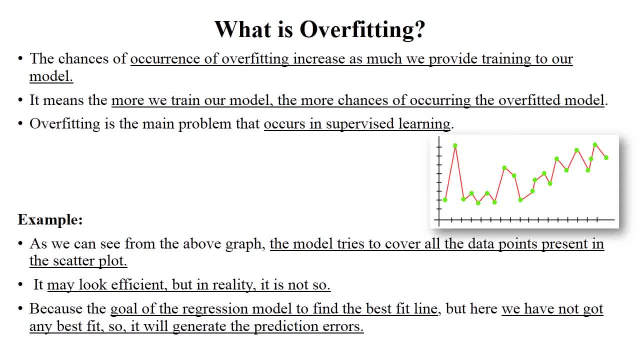 in machine learning if you train your model properly but your model not working properly at the time of testing. So this concept is called as overfitting. So chances of occurrence of overfitting increase as much as we provide the training to our model. 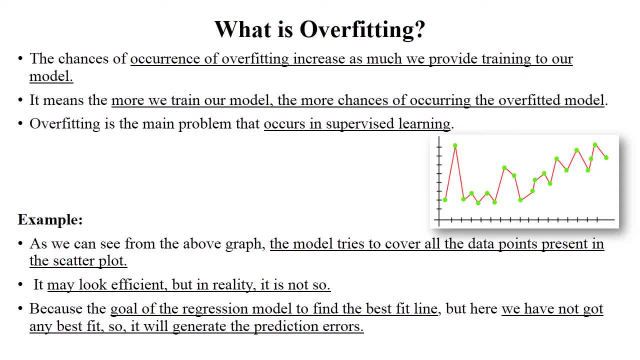 It means when we train our model, but there is a more chance of occurring. the overfitted model- So overfitting is a main problem- occurs in supervised learning. Training is properly done, but testing is not properly done, So this is a concept of overfitting. Now see: 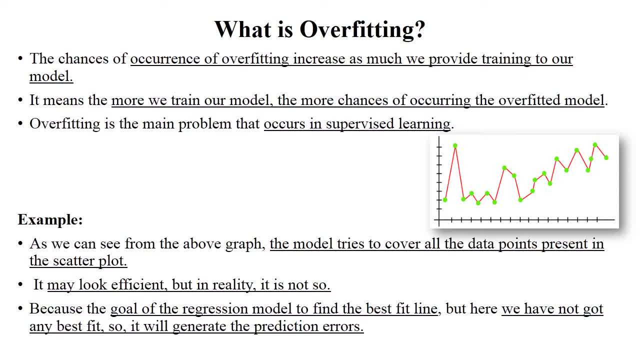 in this given diagram. what is the concept of regression? Regression: find out the best fitted line. They try to cover all the data points present in the particular graph right Here. see here in this diagram all the data points are present, that is, green colors points. 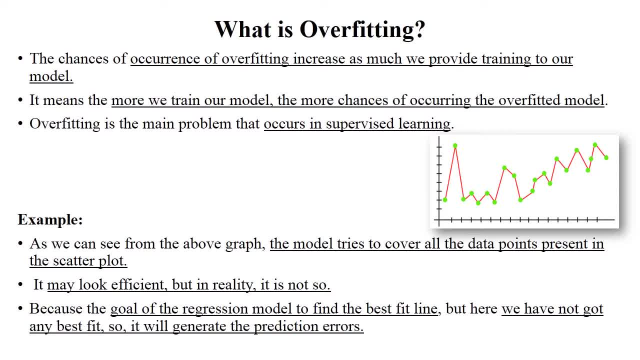 are represent at data points and red color line represent a best fit line, right? So here, best fit line. try to cover all the data points in this graph. But what is the concept of regression model? Regression model: find out the best fit line. They find out the best. 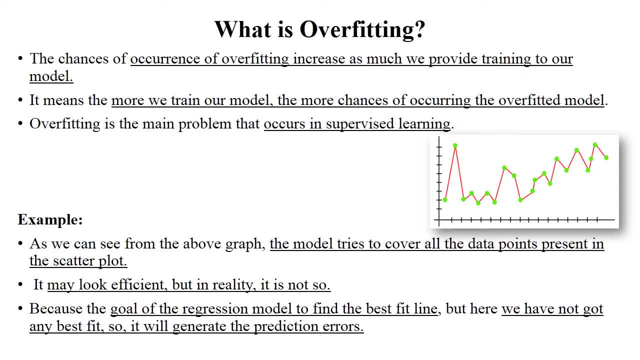 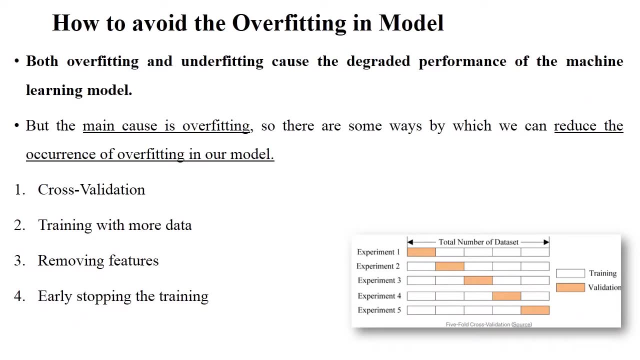 straight fit line. So here is: the particular line is not a straight one, So this is a concept of overfitting. We generate the errors and predict the errors, So training is properly done, but testing is not properly done, So this is a concept of overfitting. Now the next is how to avoid. 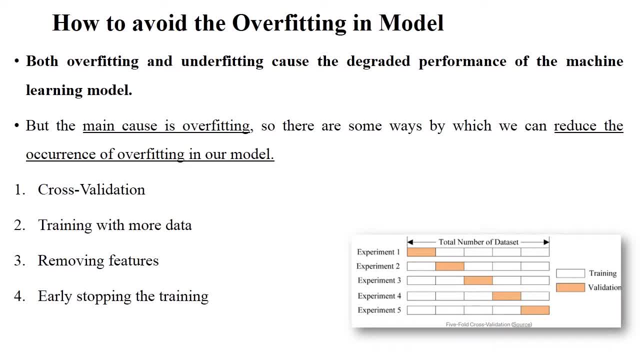 the overfitting model. So both overfitting and underfitting they cause the degrade the performance of machine learning model. So main causes of overfitting. there are some ways we can reduce the occurrence of overfitting of our model. So what are the ways? See here. 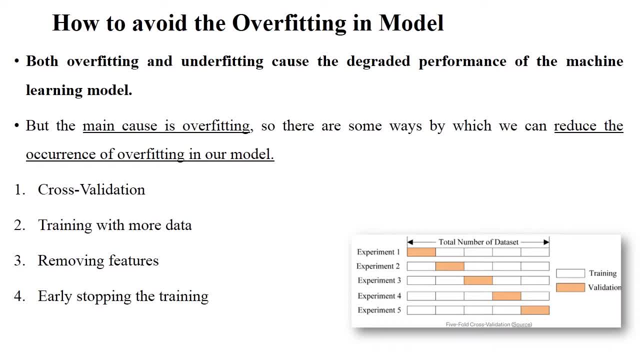 You need to perform cross validation. Training with more data means. for example, there was 100% data, is there? So use 80% of data for training and 20% of data for testing. So train your model with more data Then. 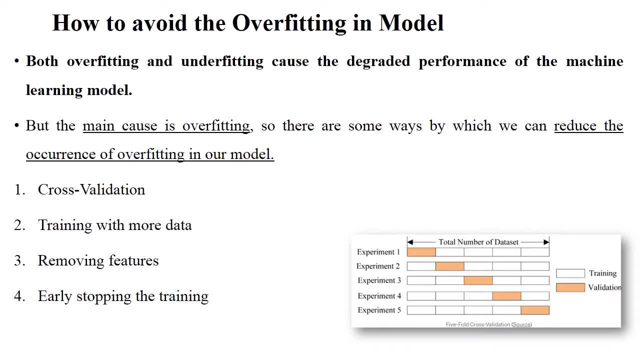 removing unwanted features. If there are some unwanted features or particular features not used for training, So just remove the features, Remove all the null values or duplicate values. So and early stopping the training and don't stop the training or train a particular model. 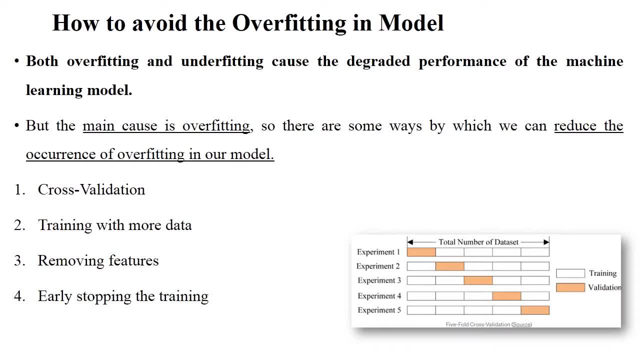 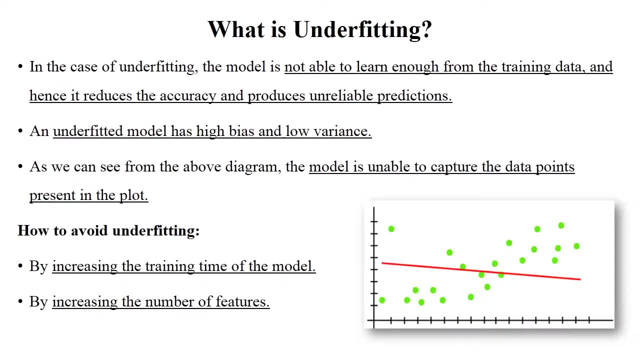 if you don't take care of your machine learning model, ok, don't stop the training procedure. So these are the some some approaches to overcome the overfitting model. Now the next concept is underfitting. so underfitting means your machine or your model not properly trained. 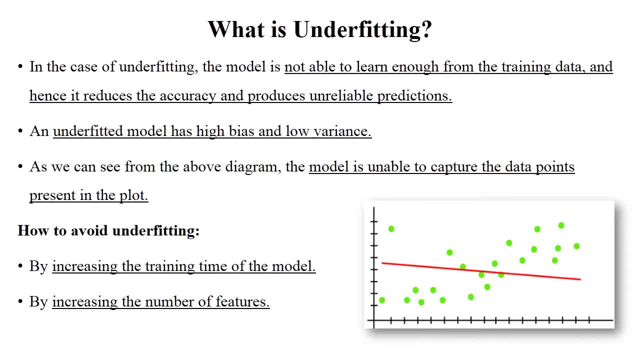 and not properly test. This is a concept of underfitting Training, also not properly done, and testing is also not so in this underfitting model, which is not able to learn the enough training data. They reduce the accuracy and reduce the prediction result. 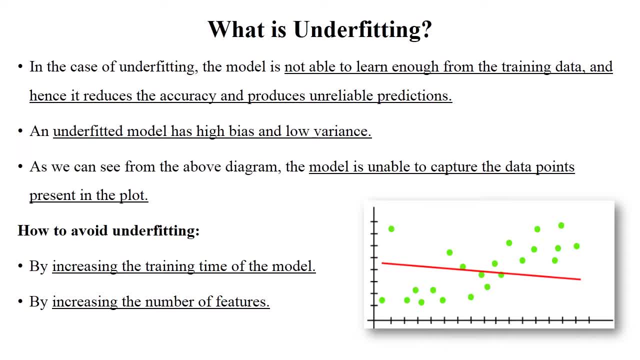 So how to avoid the under fitting? so by increasing the training time of the model and by increasing the number of features. So this, all things are used to overcome the under fitting. see here in this diagram, data points are present and best fit line is there, but data is not properly trained. because in what? 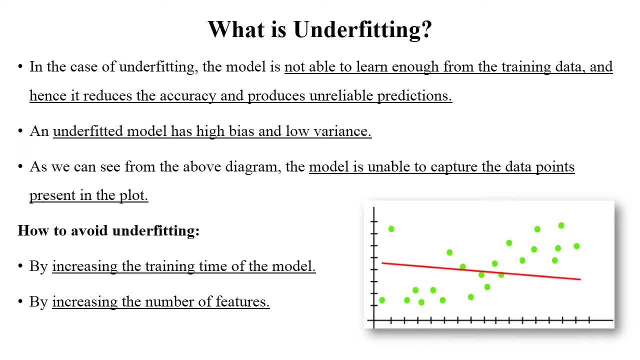 is the concept of regression. all the data points or all the actual values are just near to predicted values- This red line, are the predicted line, right, but all the points are scattered with each other and a line is also not a best fit line, right. 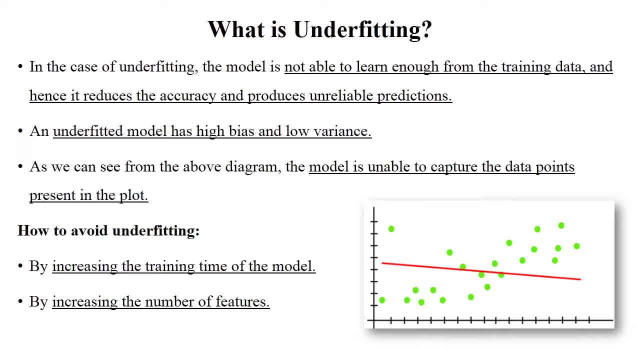 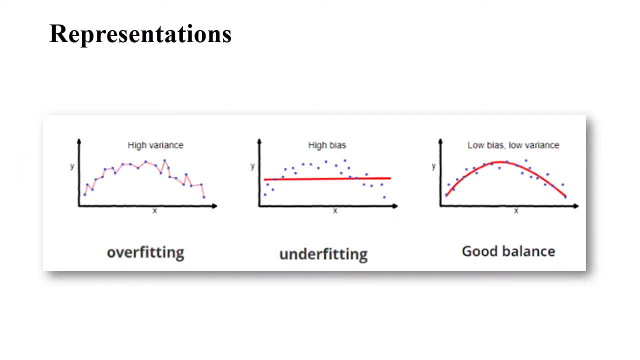 So this is a concept of under fitting, training and testing not properly done. So increase your training time and increase the number of features. Now see here: This is just representation of over fitting, under fitting and good balance. first, over fitting, over fitting means they try to cover all the points but not using best fit line. 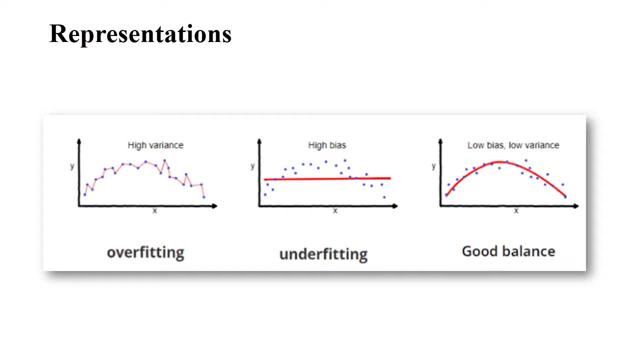 So training is proper, Really done, but testing not, and under fitting the- all the points are scatterly present and which is not a best fit line. So training and testing not properly done here and last one is a good balance. See, here This is a particular line- are present. 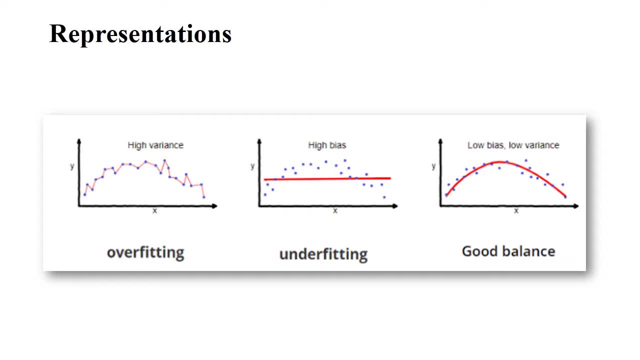 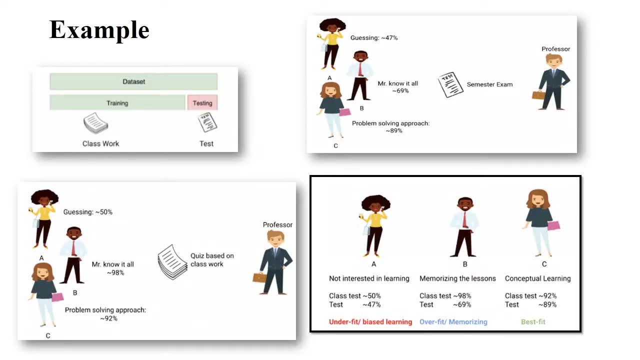 They try to cover all the points and all the data points are also properly present. So this is called a good balance. Now let's take one example of over fitting and under fitting. see, suppose, Your date. This is a particular data set. 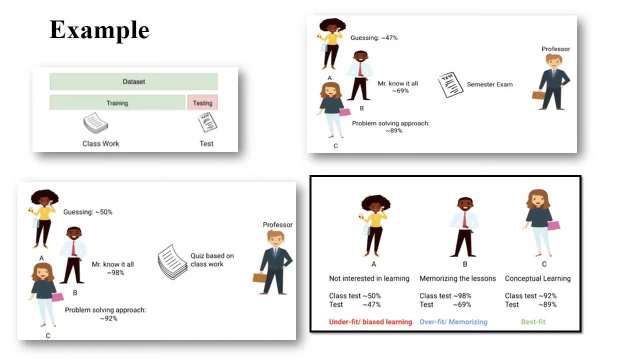 There are two parts: training part and testing part. So just consider that training part means your class work result and testing parts means your final test, final University test result. Okay, So see here in this first diagram suppose there are total three students Okay, and this two, three student in the class work, this three. 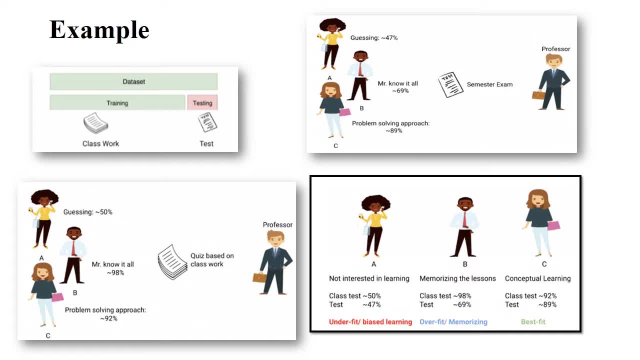 student having the particular marks: Okay. the first student use guessing approach, They having 50 marks. the second student, The- the particular student know each and everything, so they having 98% chance: Okay. and last student, that is third one. The problem-solving approach is used for solving the class test. 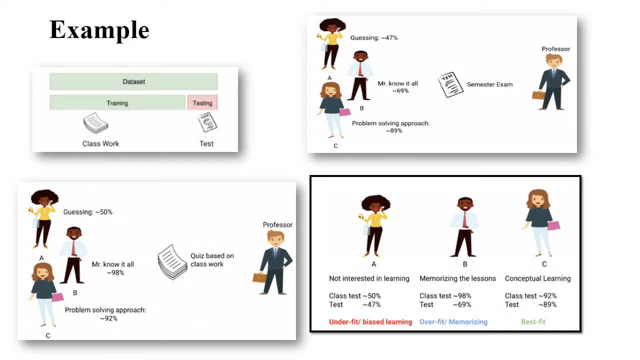 So they are having 92% marks. Okay, So according the features, they having the particular marks in class test. now third approaches in semester exam. So semester exam is for your university exam, right? So in university exam the first student also solve the paper. 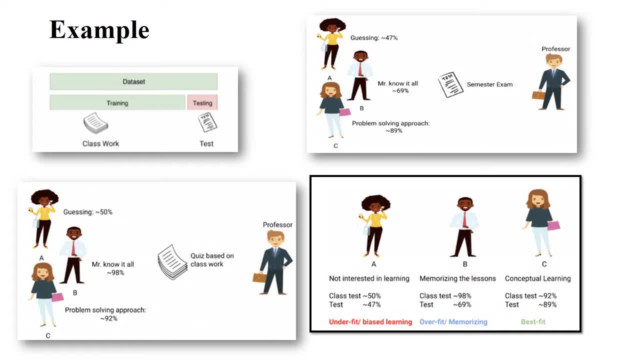 by using guessing. So, but they having 47% marks. Next, second student: They know each and everything but the particular student having 69% marks. and third student having problem-solving approach. So at that time, the particular students having 89% marks in. 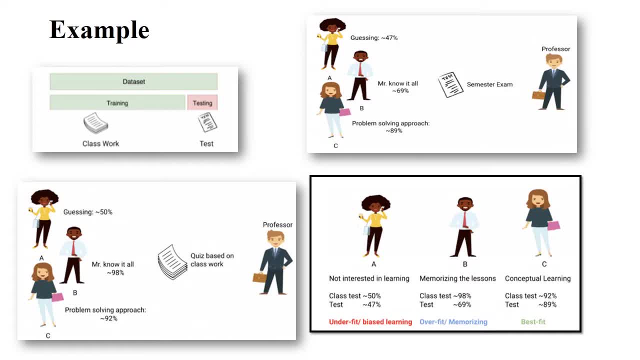 semester exam. So class test training is different and while testing the result is different. right? So what is the outcome of this example? See first, student use guessing approach. That's why the result is low, right. So class test: 50% mark. test is 47% mark. 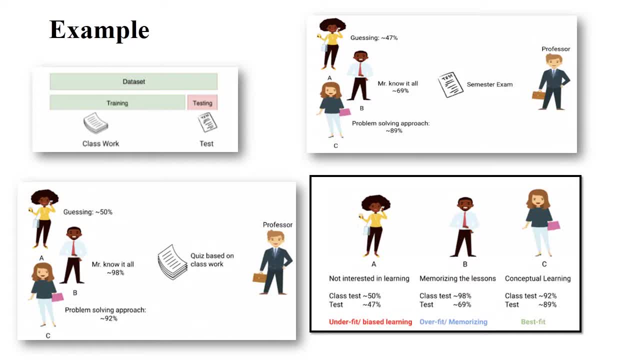 Means the particular student not interested in learning, right. So this is called as underfitting training and testing not properly done. The second student- second student- know each and everything. So at that time they memorize each and everything. they memorize the or remember the particular things in your class test and 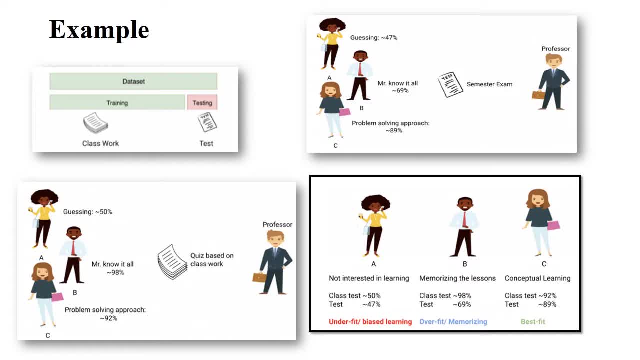 semester exam, So their class test marks is 98%, but university semester exam paper is different, So their test marks is 69%. So this is called as overfitting means: train properly but not test properly. And last one, use the problem-solving approach or conceptual. 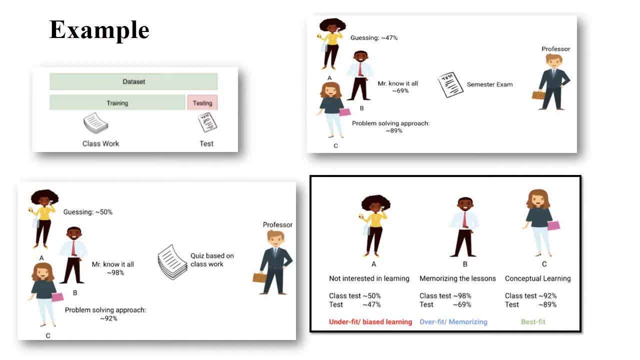 learning. So at that time their class test marks is 92 and test marks is also 89. So this is called as best fit means training and testing is accurately done. So this is just sample example of overfitting and underfitting. 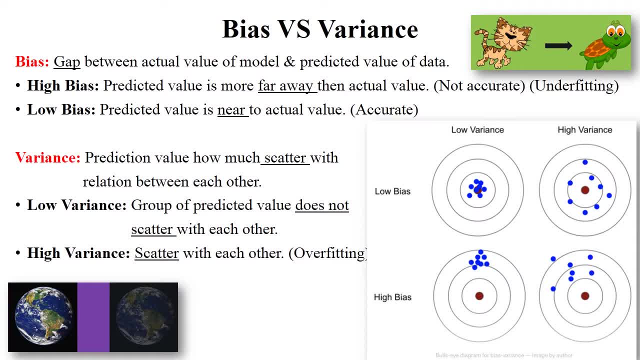 Now, next concept is bias versus variance. So what exactly bias? Bias means gap between actual value of the model and predicted value of the model. So the gap between actual value and predicted value- this is called as bias- And variance means if the data is group, present or scatterly. 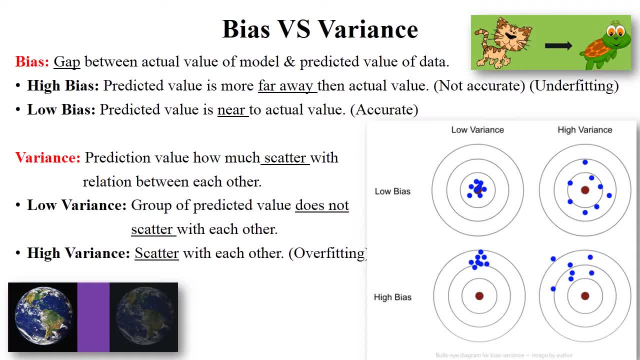 present. that will be identified by the variance. So bias has two types: high bias and low bias. high bias means predicted value is a far away from actual value and low bias means predicted value near to actual value. Okay, far away and near next variance. again has two types: low. 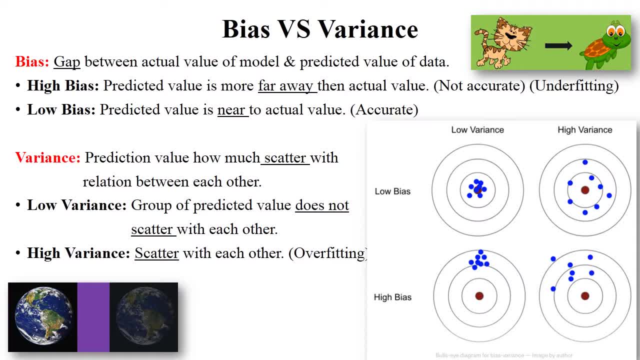 variance means all the points are not scattered with each other. means group present. that is low variance, and high variance Means all the points are scattered with each other, So this is called as high variance. Now let's see in this diagram the relation between bias and 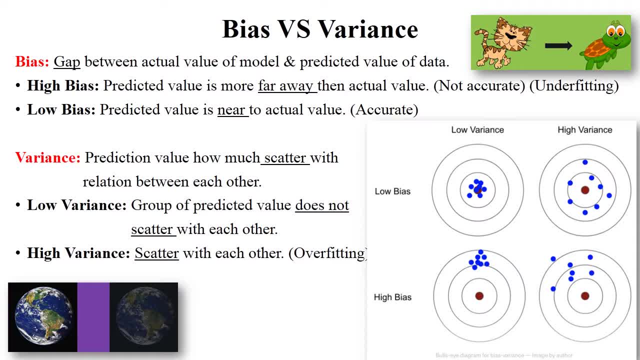 variance. see, the first one is a low bias in first diagram, low bias and low variance. So at that time your actual value is just near to predicted value, right, and all the data are present. with group, which is the other right. all the blue color data points are present in. 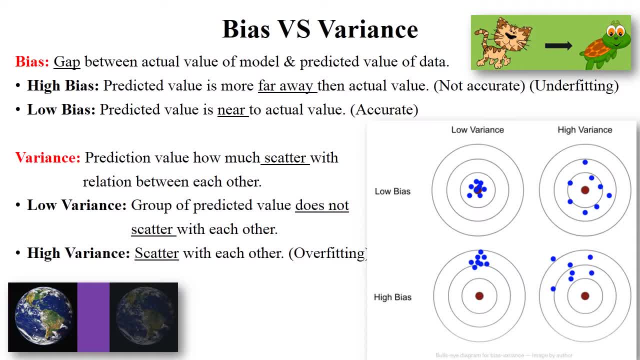 group play. So this is the highest accuracy model. They fulfill the every condition. Slow bias and low variance is the best one. Now second diagram: low bias and high variance. So low bias means actual value. blue color dots are actual value and this brown color dot is a predicted value. 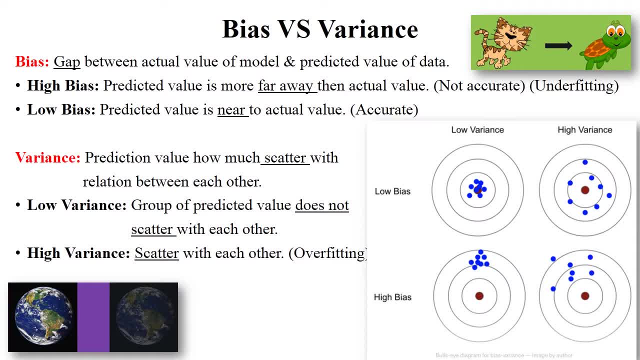 Okay, but actual value is far away from the predicted value. right and next to the high variance. high variance means all the scatter with each other. right, all the points are scattered with each other, So this is not accurate. now, third one, third one, See high bias and low variance.